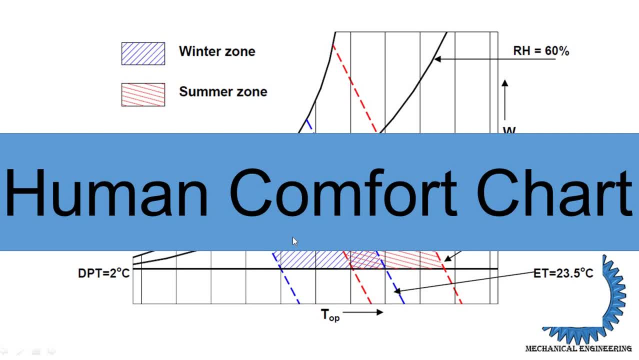 American Society of heating, refrigeration and air conditioning engineering. they are collecting the number of people's they are sitting on, to the different temperatures, in different relatively humidity, and some people are feeling comfortable, some are not- and collecting their data and after collecting their data, they are making the one charge that is known as the human comfort charts. so in this they 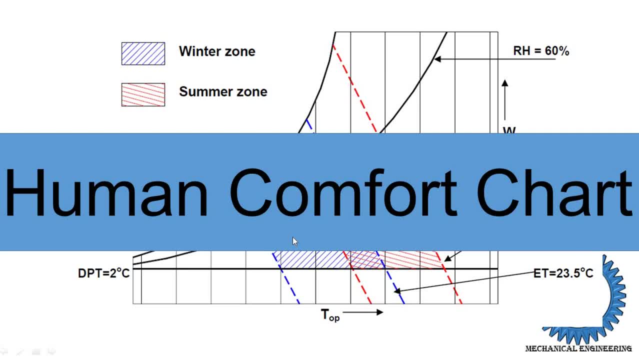 are changing the three parameters: temperature, relative humidity and air motions. so we are combining these all. the factor then it is known as the effective temperatures, okay, and the air velocity is set 5 to 8 meter per minute. velocity and dry bulb temperature is changed. wet bulb temperature is changed, which is recognizing stories. power now we find more rising or not raising to minus 5 meter per minute. velocity and dry bulb temperature is changed. the air would get less. energy of air will remain faster as we get larger than the hyung of Crossing frequency. then this Esper model is set to several factors and these are referred to the ester balls and cooling resources. so if both of them are completely the same will never get away from those things. but the quality of the four- Medic voulais complex. on, 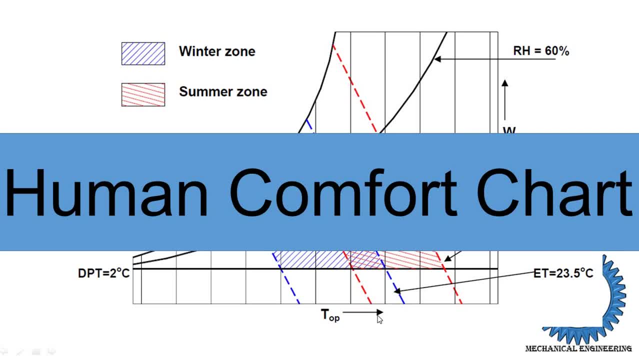 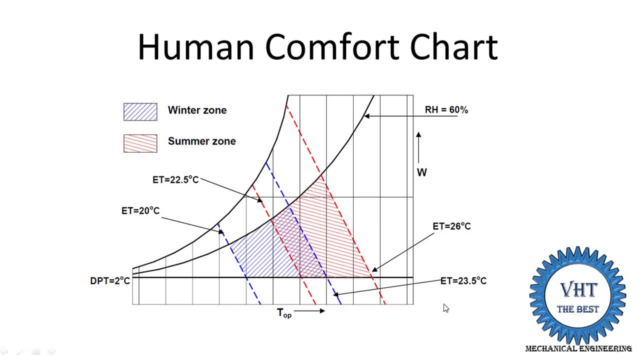 bulb temperature is changed for the certain regions of times. okay, and it is plotted on one graph and i completely show you the graph here. so it is a graph of effective temperatures. effective temperature means it is a combination of dry bulb temperature, wet bulb temperatures and the relative 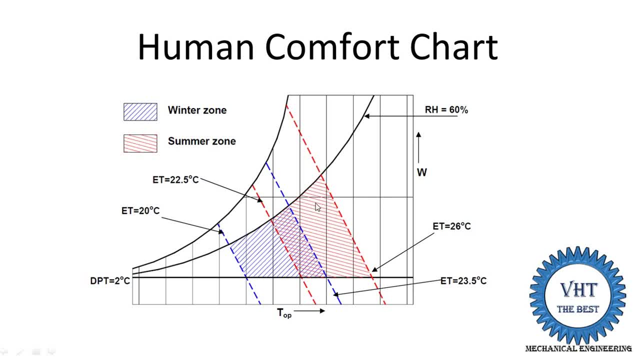 humidity: okay. now this relative humidity is comfortable between the 30 to 70 percentage. okay, so 30 below the 30 percent relative humidity, the screen skin becomes too dry and relative humidity: if increase about a 70 percentage, then skin becomes too sticky. that's why the 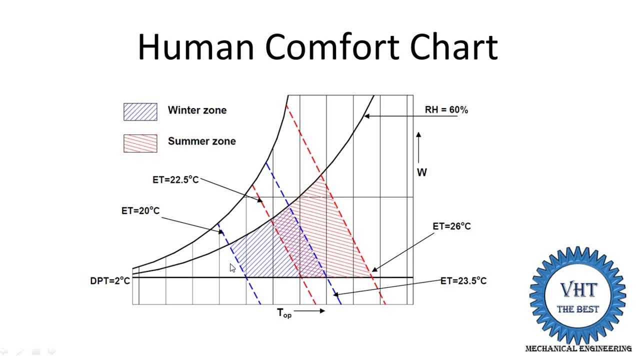 relative humidity is between the 30 to 70 percentage in the both the condition for winter and summer zone. now first we focus on to the summer zone. okay, so in this summer zone there is a red color line is indicate if the comfortable zone for the human being, this red line is indicate the 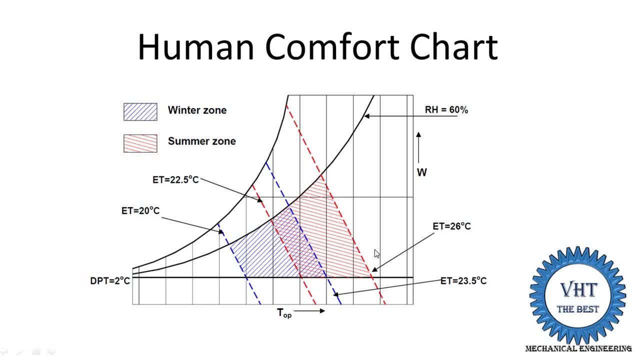 effective temperature of 22.5 degree centigrade and another red line is indicate that 26 degree centigrade. so during the summer season the person is feeling comfortable at the effective temperature of 22.5 degree centigrade to the 26 degree centigrade and what is relative. 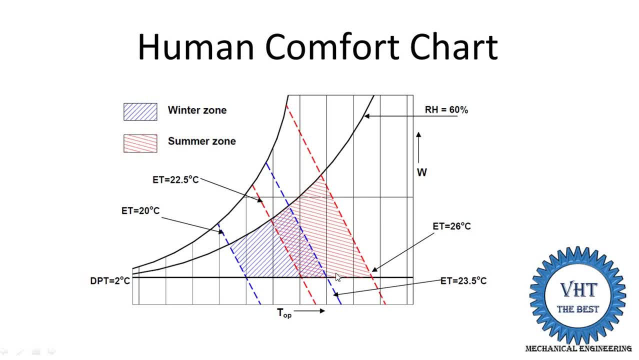 humidity is between 30 to 70' these line of the humidity, here the line is humidity for the 30 degree and these line of humidity is for the 60 degree. ok, so these red zone is indicating comfortable range for the summer seasons. ok, so all the person are not feeling. 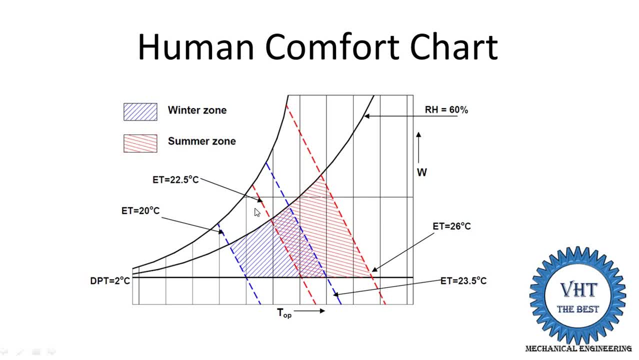 comfortable at the one specifc effective temperature. ok, some are feeling effectively at the 22.5 degree centigrade. some people are feeling effective at 26 degree centigrade. ok, so we are not comfortable at this. are saying that at that 24 degrees centigrade all the people are feeling comfortable because it is. 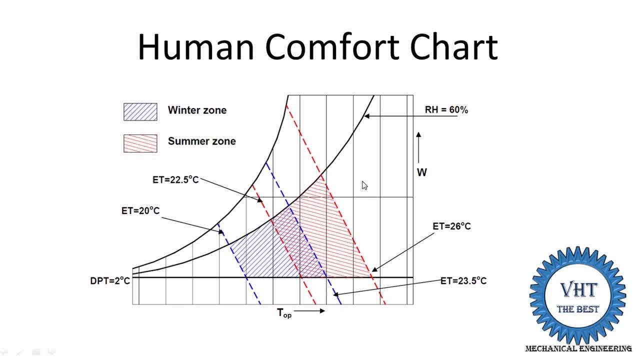 depend upon the psychological conditions of the human being. that's why its range is change. now we study for the winter zone. for the winter zone, the 90 percent of the people is feeling comfortable at the effective temperature of 20 degrees centigrade. so this blue line is indicating: 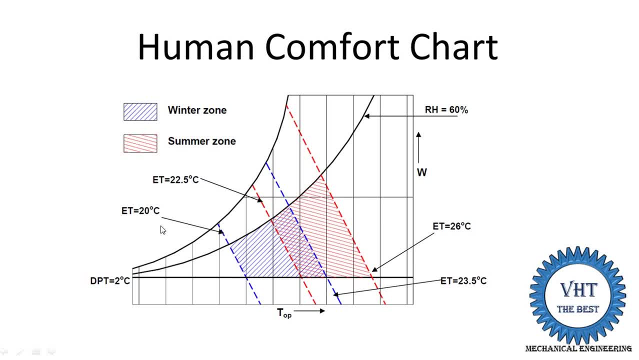 the effective temperature of 20 degrees centigrade means at 20, 90 of the people is feeling comfortable. that is research done by the astray that collecting the data- and another 10 of the people are feeling comfortable between the 20 degree centigrade to 20. sorry, it is a 23.5 degree. 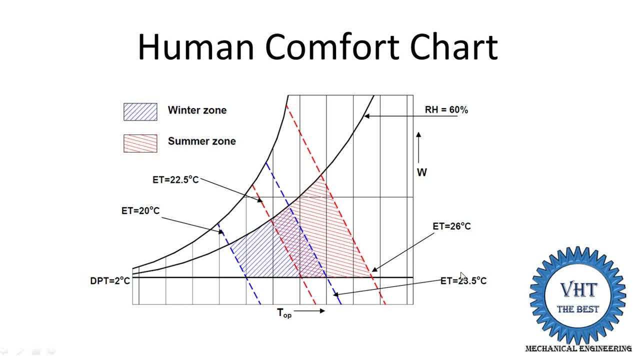 centigrade, so it is another blue lines. it is a 23.5 degree centigrade, so it is a range of 3.5 degree centigrade effective temperatures for feeling the comfortable in winter, okay, and also the for the summer seasons. it is a 3.5. 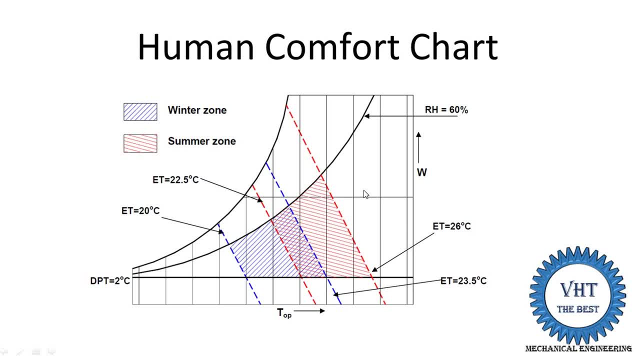 because 26 minus 22.5 means it is a range of only 3.5 degree centigrade for feeling comfortable. so this blue zone is indicating the comfortable zone for the winter seasons. ok, now here we see that winter and summer zone is mixed with each other. ok, so it is. 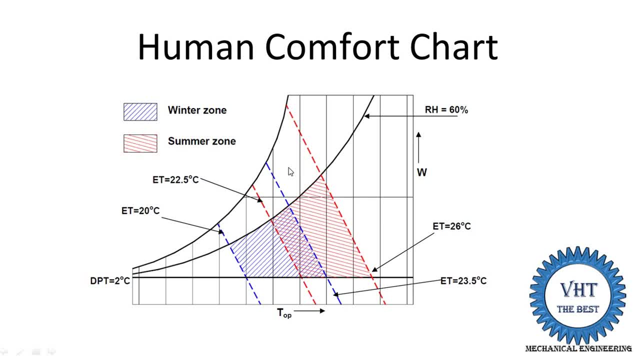 a 22.5 degree centigrade, and 23.5 degree centigrade means this is a 1 degree effective temperature range. on that people are feeling comfortable in both the seasons, either in the winter and either in the summer. ok, so it is a range of effective temperature: 22.5 degree centigrade. 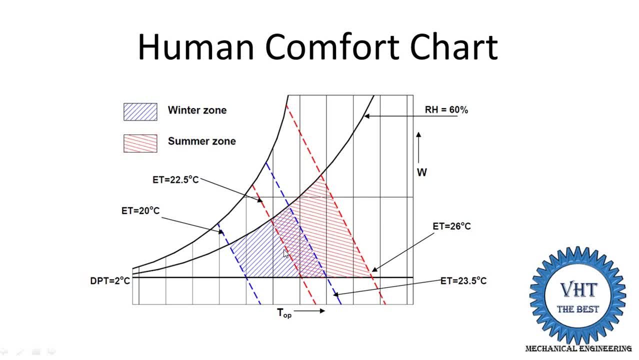 and 23.5 degree centigrade on this region. some people are feeling comfortable in both the season, as well as winter or in the summer. ok, thank you for watching this video. if you learn something, then like my video, subscribe channels and share with your friends.